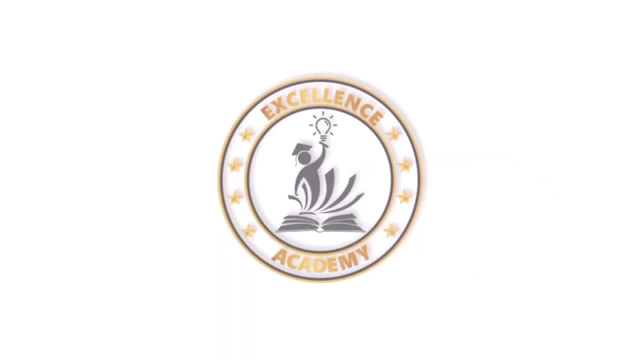 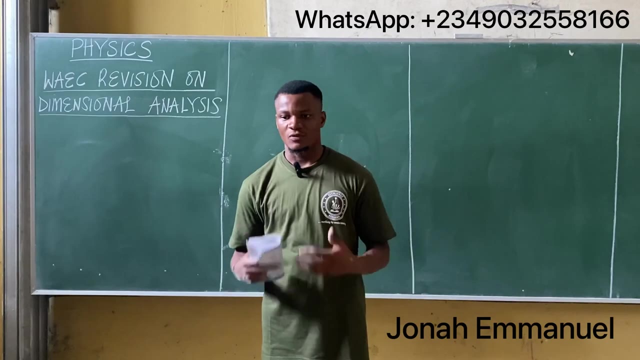 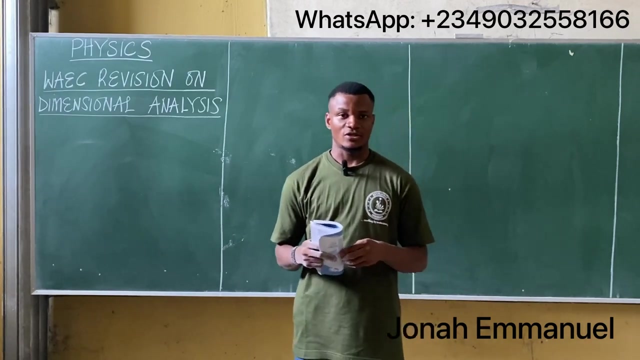 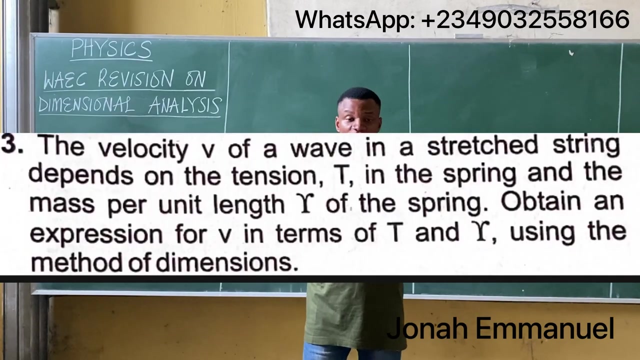 Hello and welcome to today's class. For today's class we'll be looking at Weier's physics question on dimensional analysis. We're trying to solve some Weier's questions on dimensional analysis. Now this question here says the velocity v of a wave in a stress string. 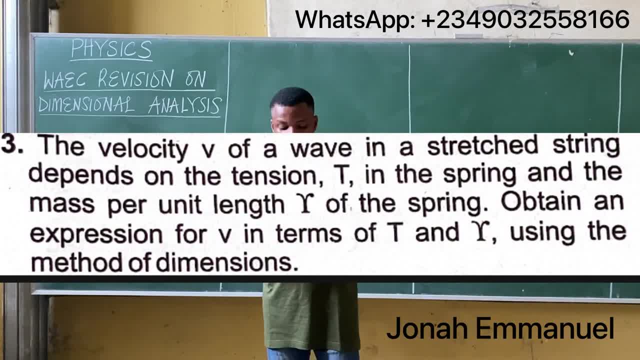 depends on the tension- t in the string- and the mass per unit length. you have that symbol there. that's gamma of the spring full stop. Obtain an expression for v in terms of t- that's the tension, and gamma- that's your mass per unit length- using the method of dimensions. 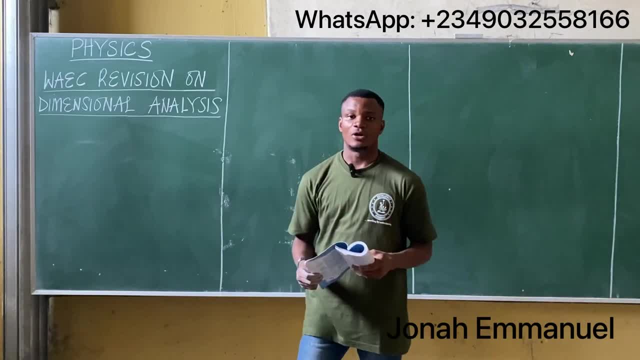 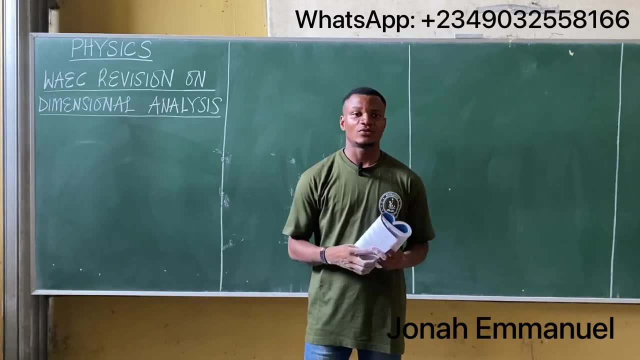 All right, let's get this done, please. So this is a question on dimensional analysis. How do we solve this kind of question? Now, the first thing you have to do is to write out the given parameters. The first thing there says the velocity of a wave. So the first parameter. 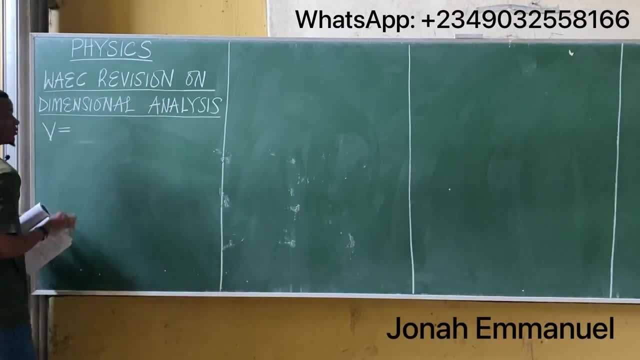 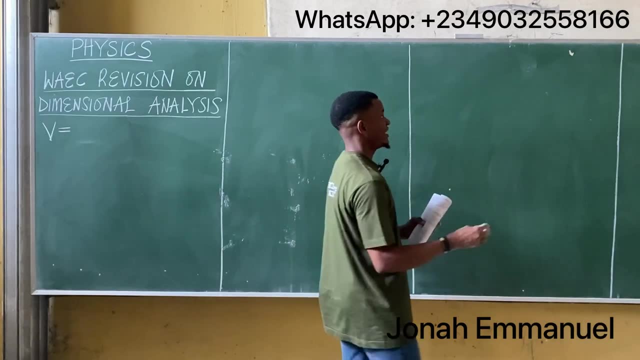 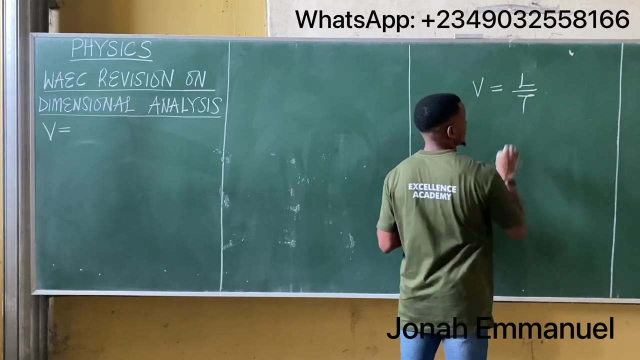 given there v velocity, that's equal to the dimension for velocity, the dimension for velocity. Now, what do we know? We know that velocity v is equal to displacement, which is a length all over time, that's t. 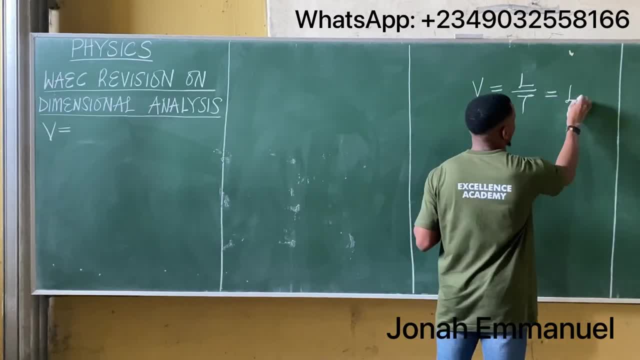 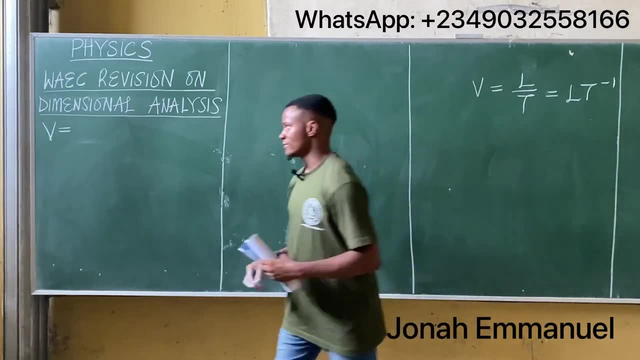 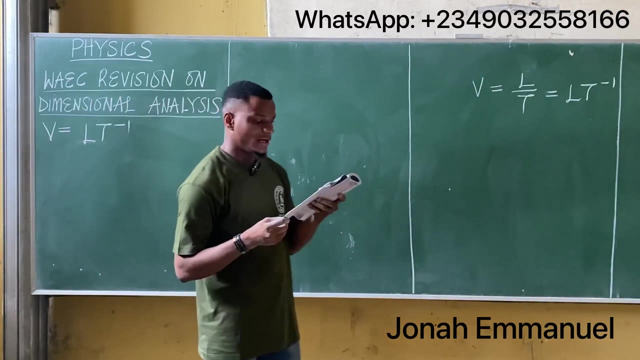 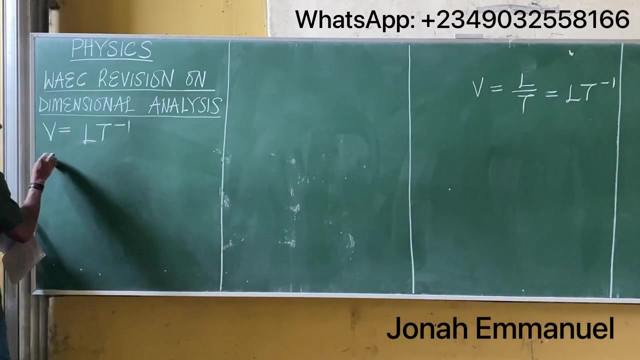 If you write this one here in index form, it's equal to l t to power minus one. This becomes the dimension of velocity. So hence v is equal to l t to power minus one. Next episode of a wave in a stress string depends on the tension. So the second parameter given there, tension t. 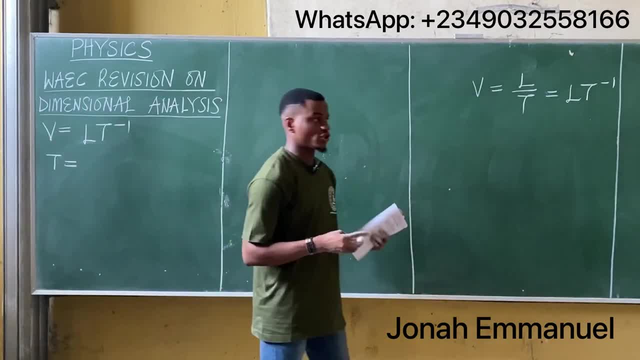 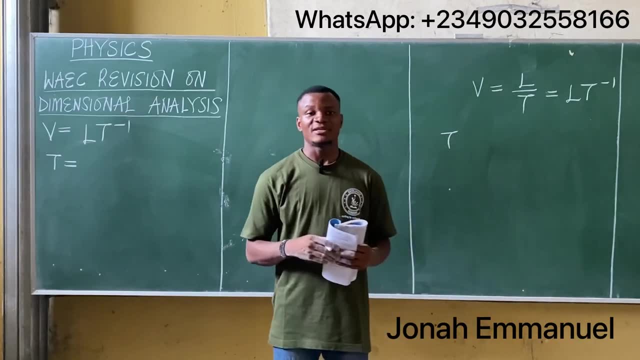 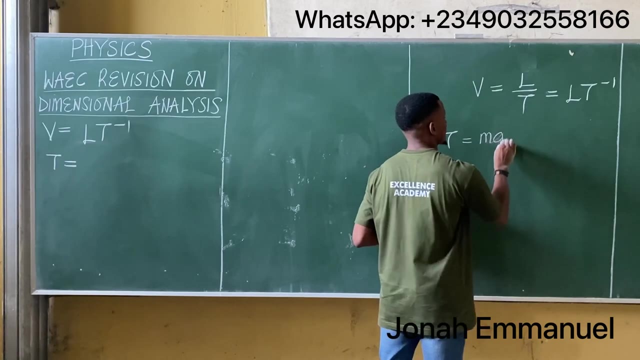 is equal to. let's get the dimension for tension. Tension is simply the force that acts on a stress string, So hence it means that tension and force has the same dimension. I know that force is equal to mass times acceleration, So that's true. 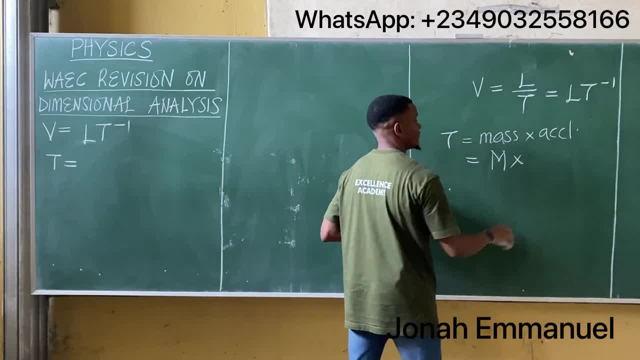 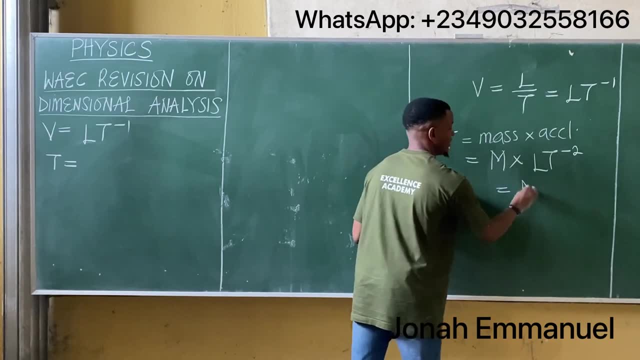 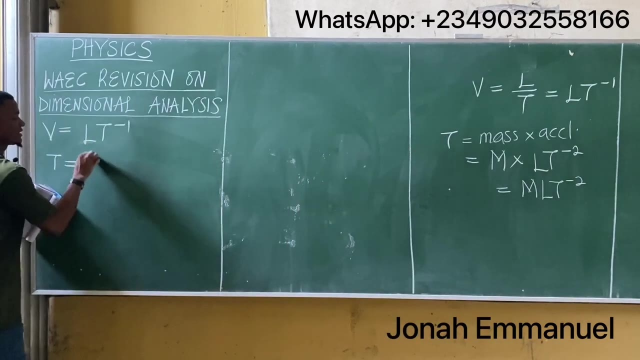 Dimension for mass is capital. M times for acceleration. the dimension is l? t to power minus two. If I combine this, I'm having m? l t to power minus one, So that's true M l t to power minus two. So I'm having dimension for tension as m l t to power minus two. 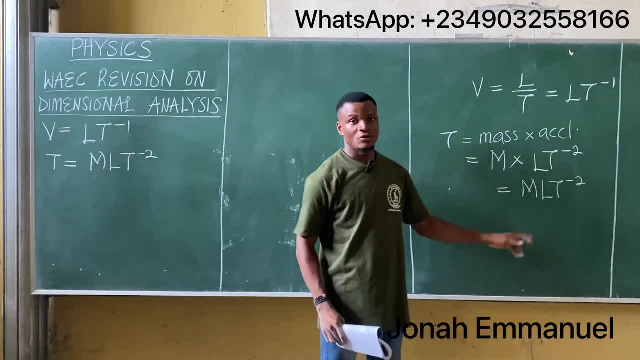 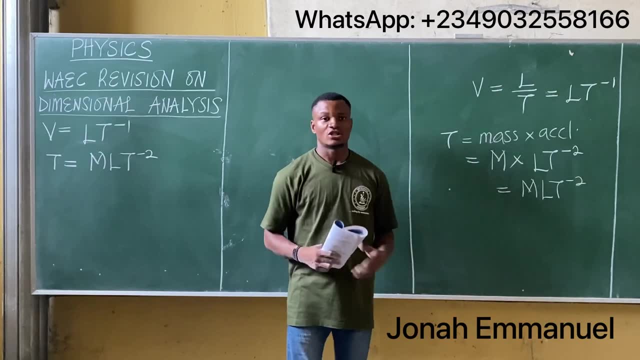 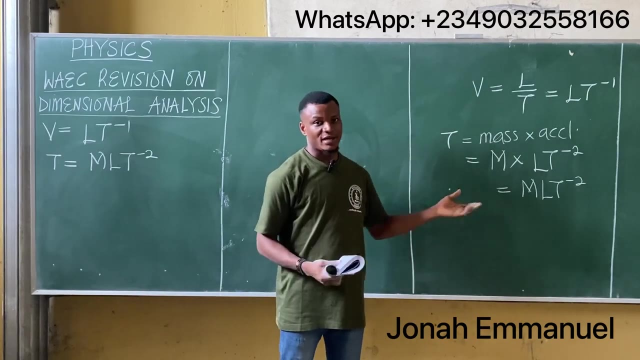 By the way, if you don't understand how we got to these things here, we've already treated this in a previous class, So if you want to get the full tutorial video on how this works, just simply check the description of this video. I'll leave a link to a full tutorial course on dimension. 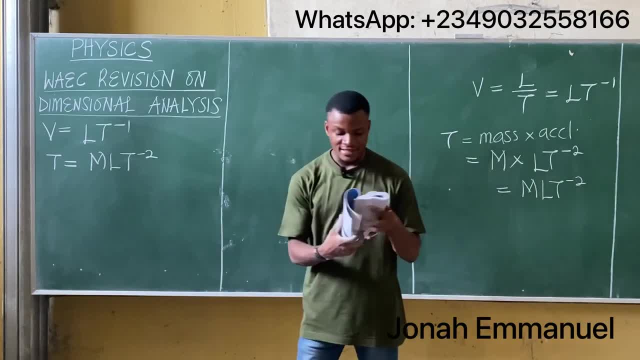 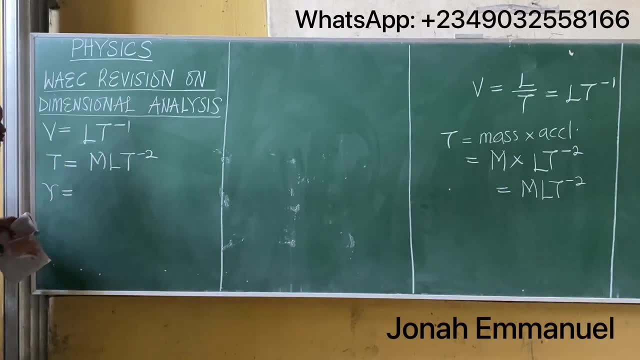 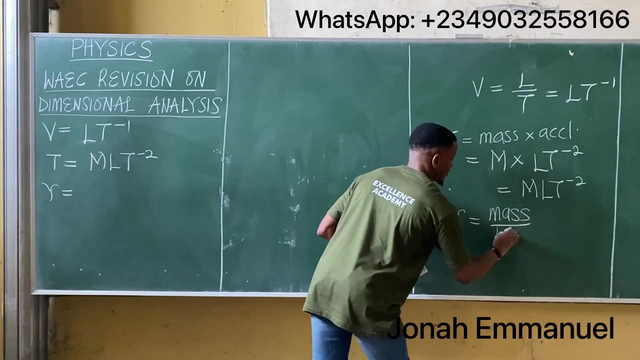 All right, let's continue with this. This is mass per unit length, which is gamma. So they give us gamma here as equal. to now we are told gamma has been equal to mass per unit length means mass over length. Mass is capital M length. 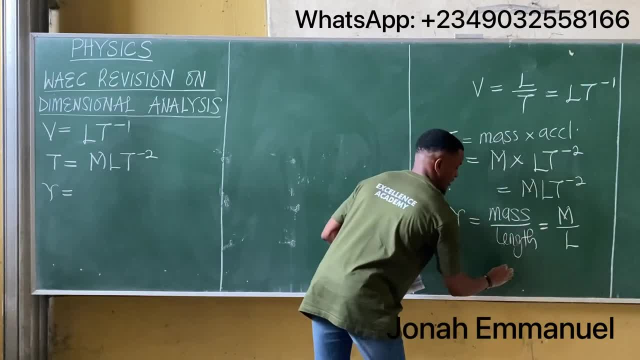 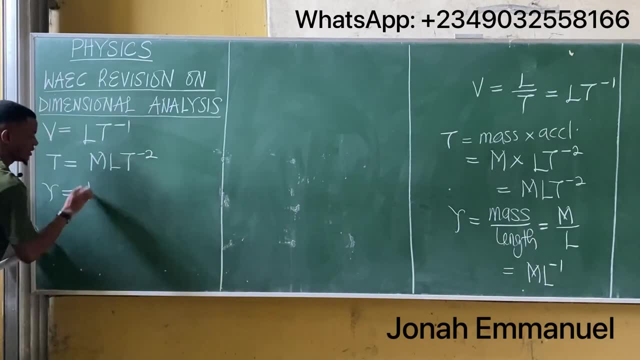 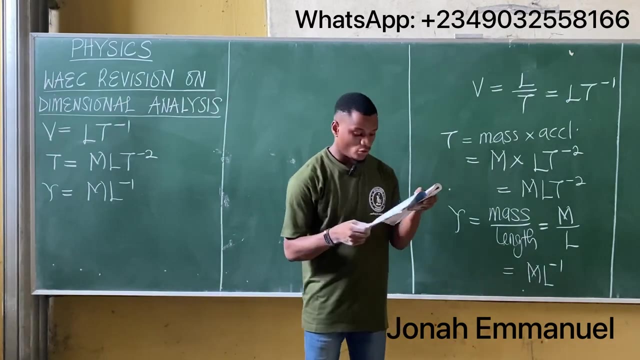 is capital L. If I write this in index form, that's equal to m? l to power minus one. So my dimension here is m? l to power minus one. All right, I think that's all the parameters we are given here. 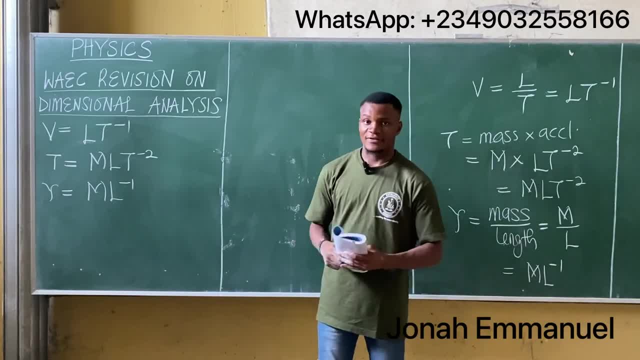 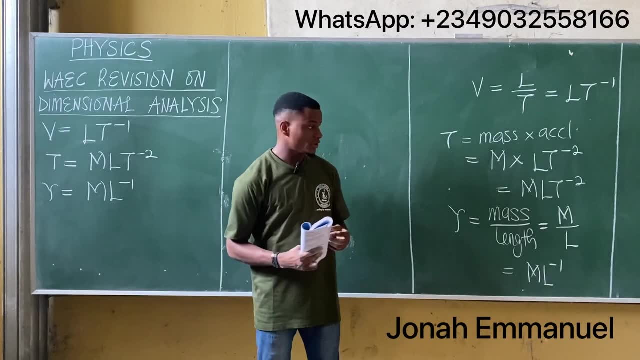 All right. so if so, we can now proceed to solving this. So I've said, if you don't understand how we got this one here, we've discussed this in our previous classes. I'll leave a link to the description. I'll leave a link to the tutorial video on dimensions and dimensional analysis. 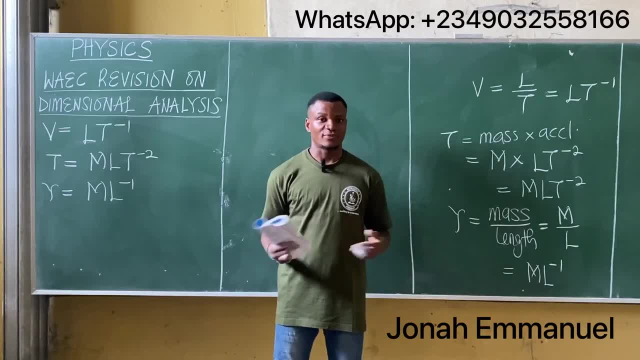 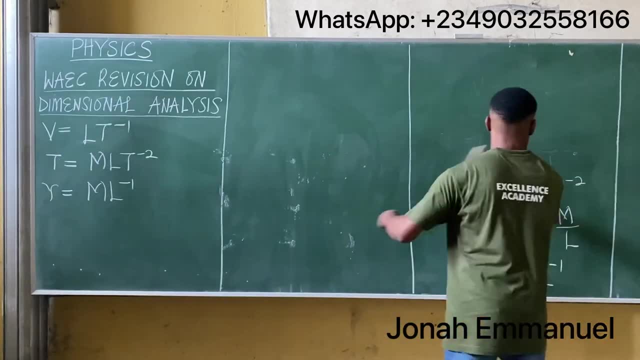 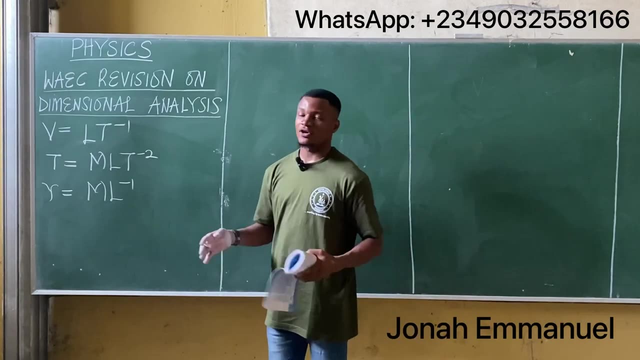 in the description of this video. So just check the description. You'll see the link to that full tutorial class. Let's proceed with this. All right, so our next task here says: after getting to your first task when it comes to: 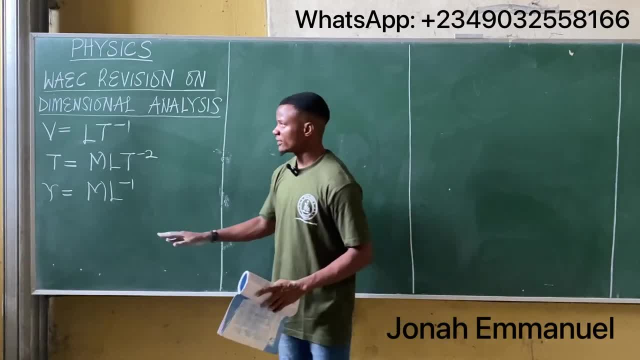 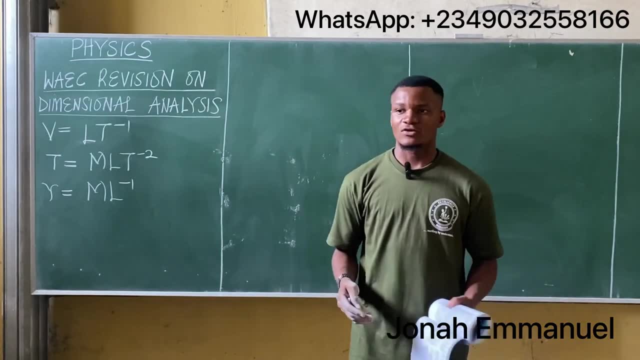 questions on dimensional analysis is to get out the parameters given and their dimension. So after getting this out, what next? Next up, you have to look for that particular parameter in which other parameters depend upon. To get that parameter, you have to look for the parameter. 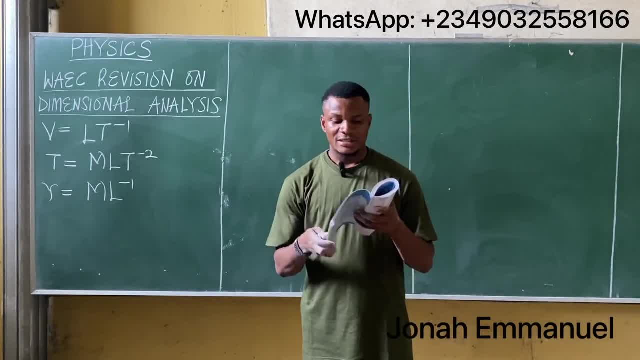 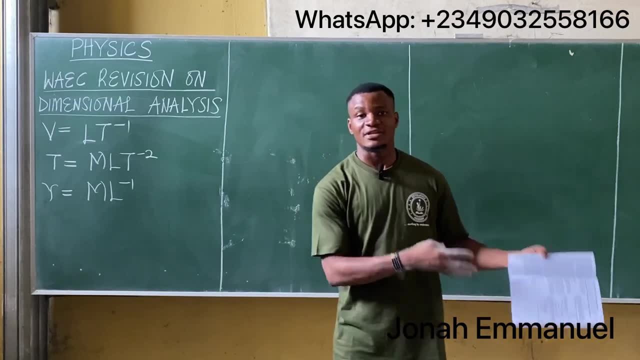 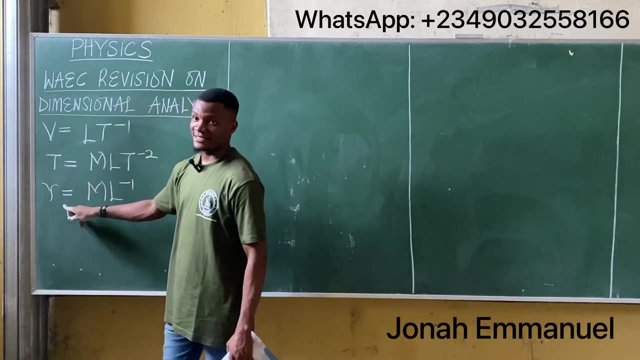 you have to read your question carefully. Now check. The question says the velocity of a wave in a stress string depends on: so it is the velocity that depends on others. So if that's so, it means that velocity depends on this and this. To write: dependency in mathematics. 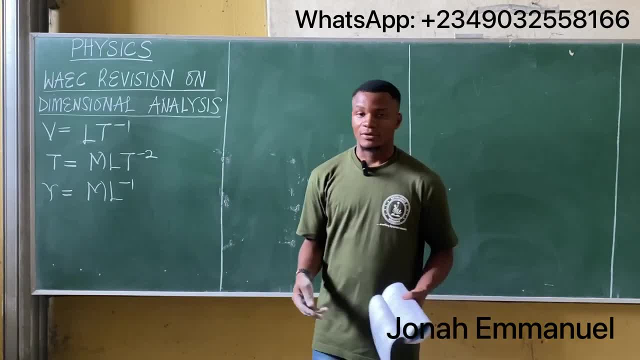 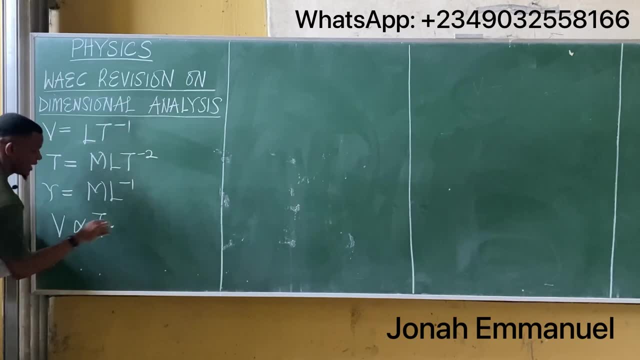 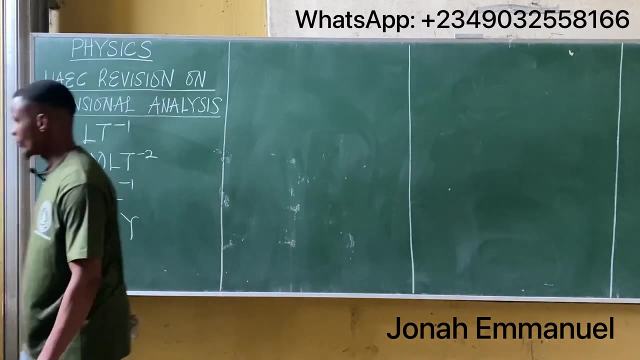 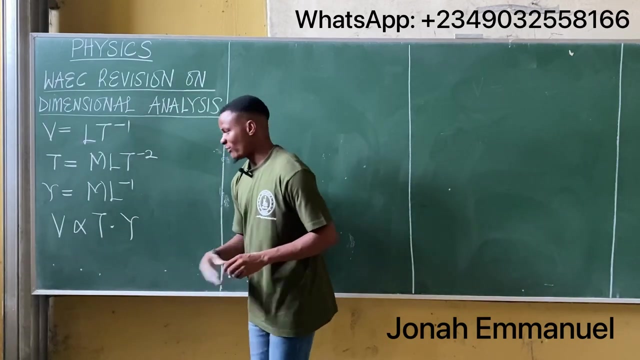 we use directly proportional. okay, So that means velocity is directly proportional to tension- this- and mass per unit length- this, All right. All right, so I'm having this because velocity depends upon the tension and the mass per unit length. At this point, what next do we do? 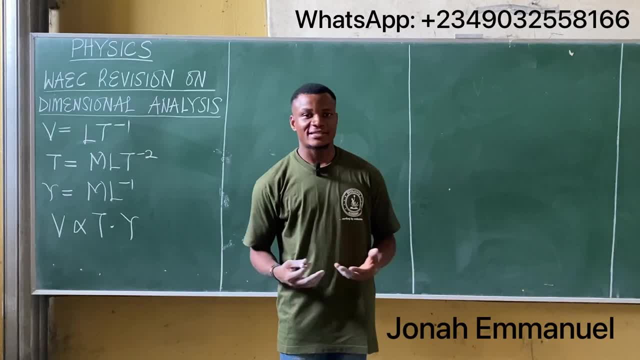 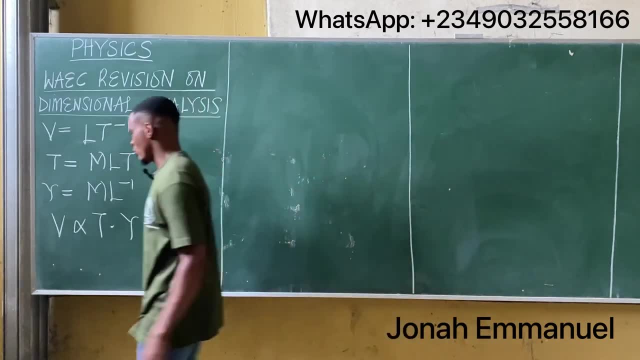 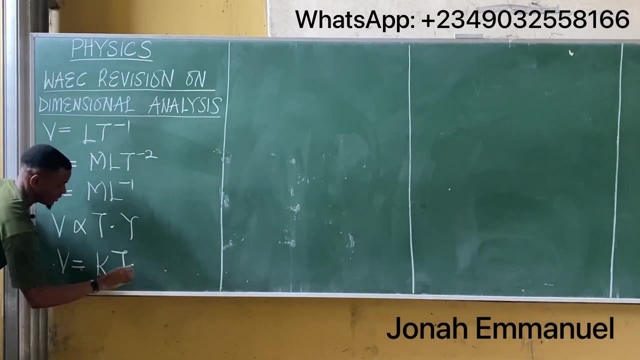 We have to take this off. To take off proportionality sign in mathematics, we said you would replace it with equal to and add a constant. So replace this with equal to. I have that V is equal to add a constant k, and then t dot gamma. This is gamma, not y. It's called okay. 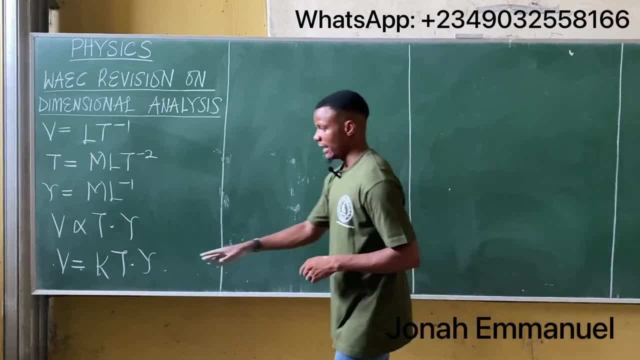 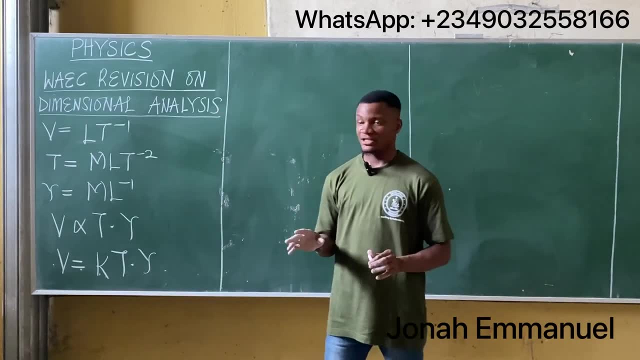 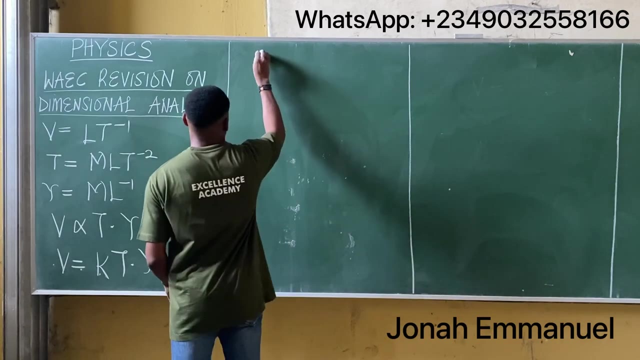 Gamma dot y. So what next? At this point, assume the tension. sorry, at this point, assume the constant to be 1, all right, So it's more like saying: you can ignore the constant here, So I'll ignore the constant and just work with this one here. So it means that V is equal to. 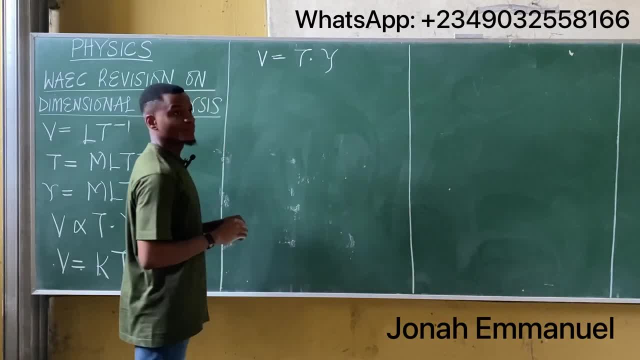 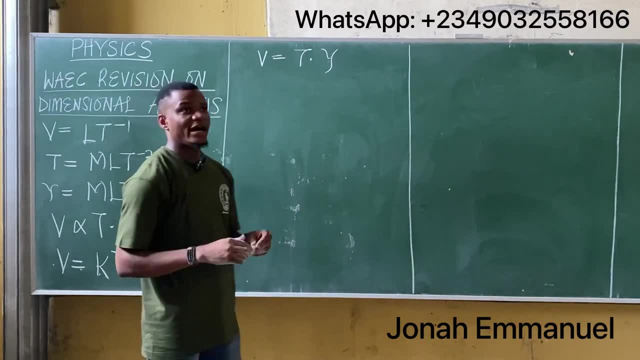 c dot this. So I have this Okay. So what next? here At this point? now, all right. So at this point, what next? You would add: what's it called Superscripts? The superscripts here would be x. 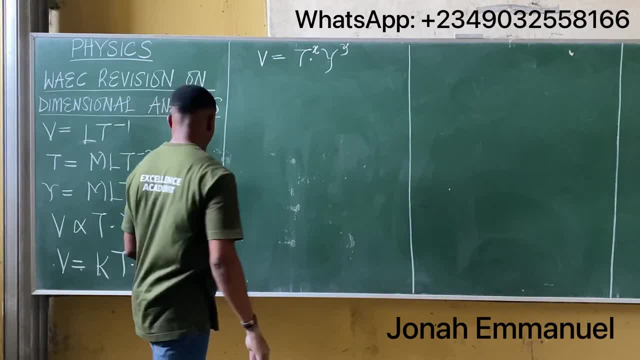 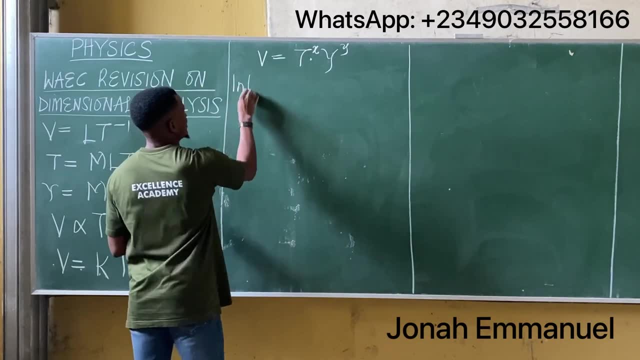 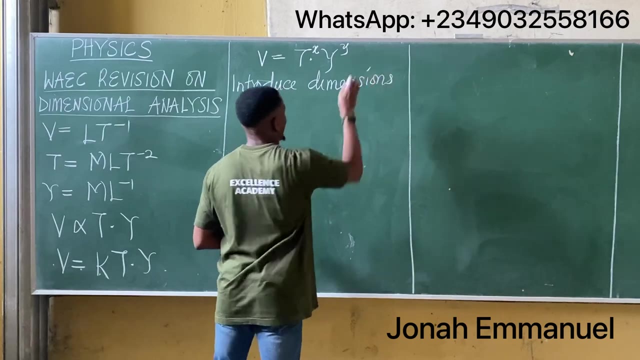 here would be y. So these are the steps. okay, After you ignore constant, you add superscript to this: x and then y. At this point now, I will now introduce constants, sorry, introduce dimensions. I will now introduce dimensions For V. my dimension is l t to power minus 1. 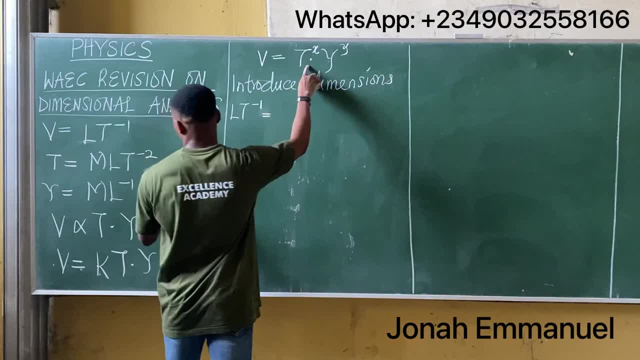 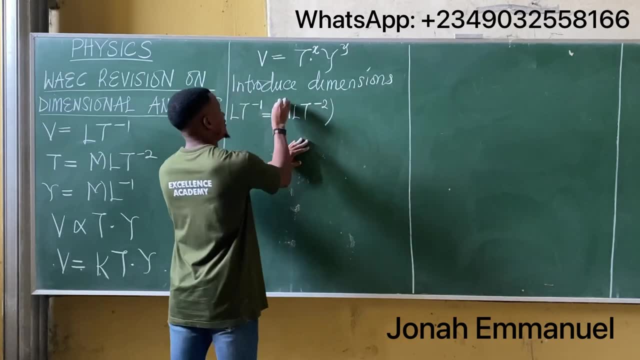 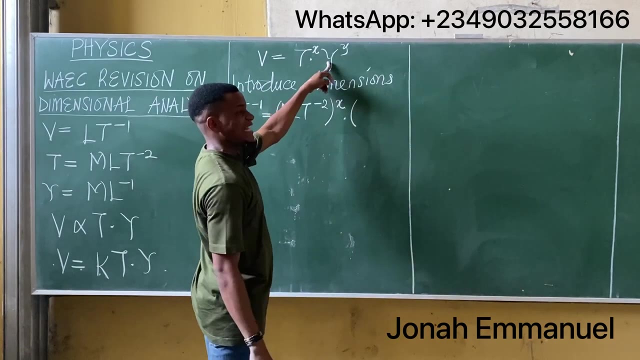 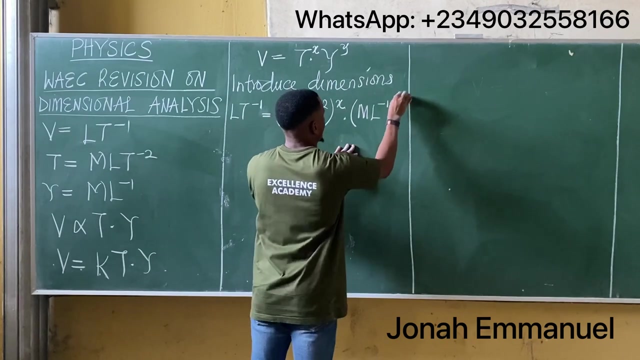 is equal to for t. my dimension is m, l, t to power minus 2.. All of this takes this power here, which is x, dot for gamma or mass per unit length. you can see. dimension is is m, l, t to power minus 1, and then y. So we have this All right. So dimension for 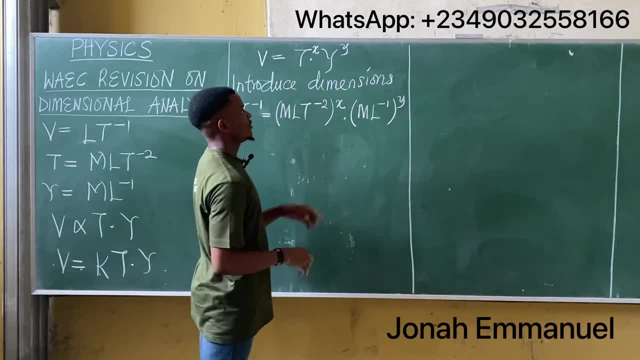 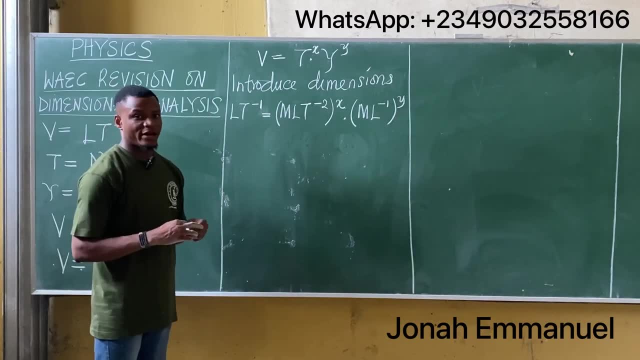 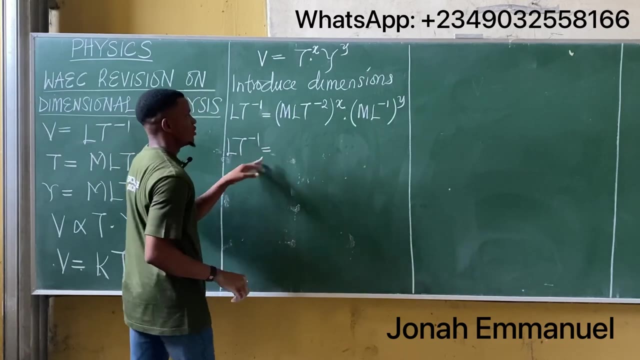 tension. is this: l t to power x. Dimension for mass per unit length. is this l t to power y. So at this point, what next? I will expand my bracket. So this becomes here: is l t to power minus 1 is equal to multiply this m to power x. It becomes m to power x and then y. So this: 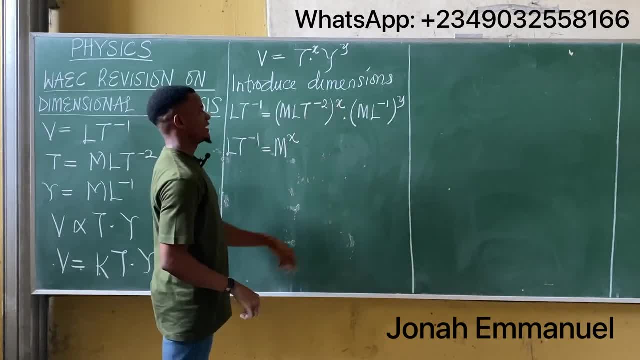 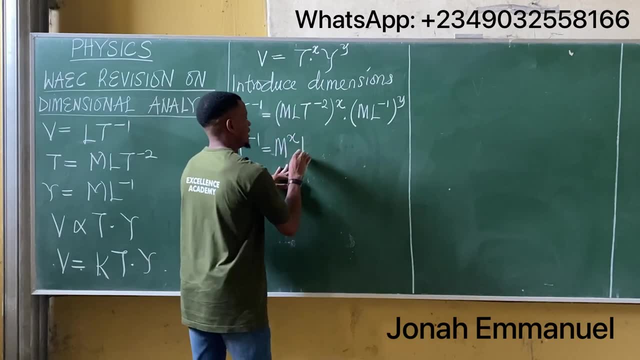 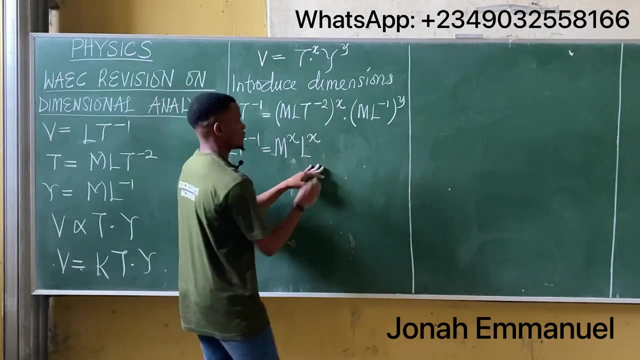 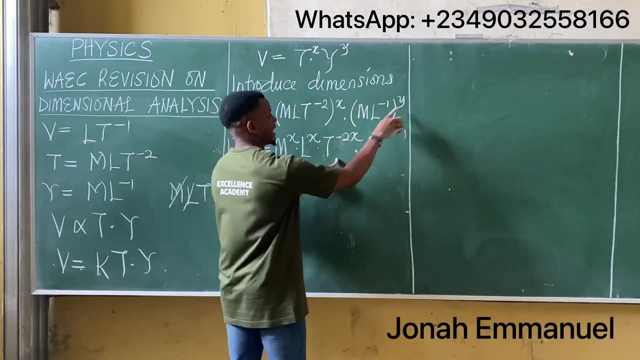 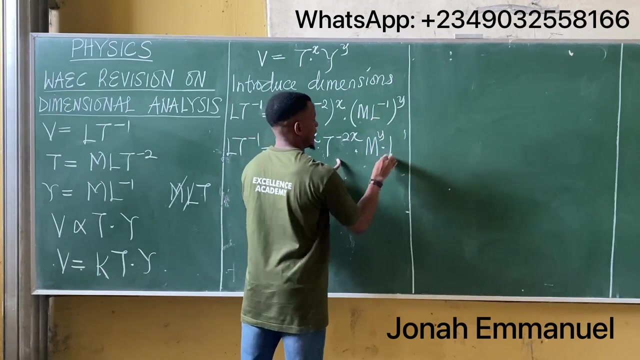 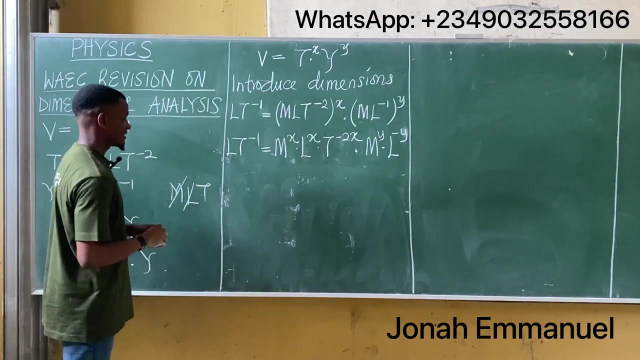 gives me a value of m t to power minus 1.. So my Kirchner expression- here is my dimension- is m times L times minus 1Y gives you L minus 1 times Y is minus Y. So I have this Alright. my next task is to: 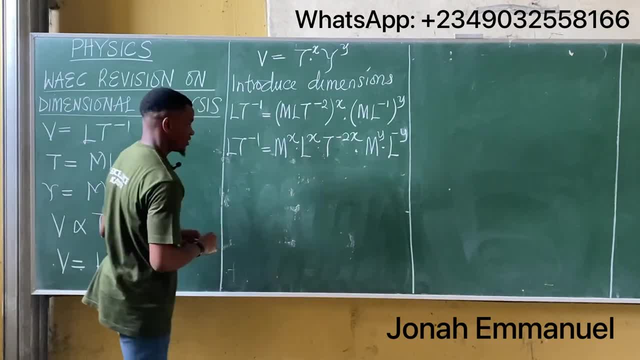 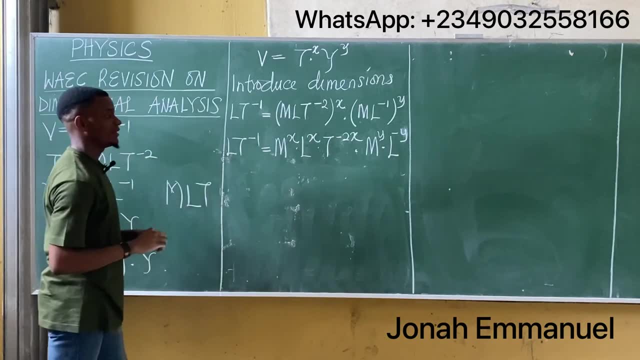 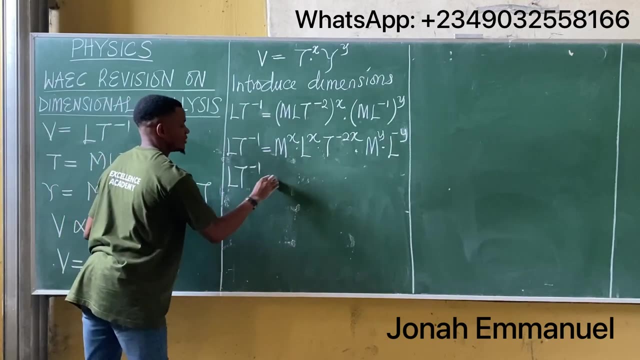 Alright, so my next task is to rearrange this in terms of M, L and T. Rearrange this one here, the right hand side, in terms of M, L and T. So I have L T to the power minus 1 is equal to. 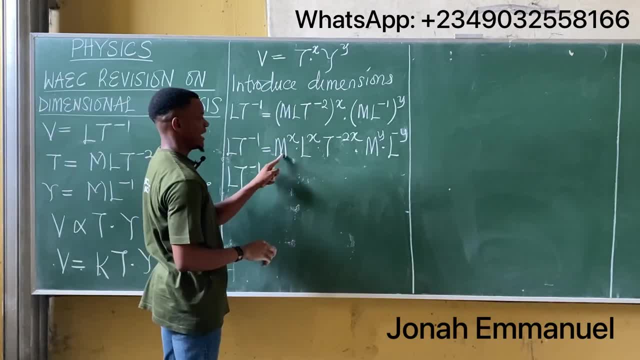 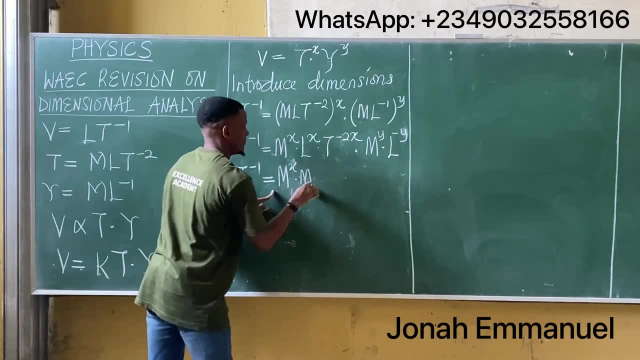 take the M's first. So I have 2M here: M to the power X and then M to the power Y. So it becomes M to the power X, dot M to the power Y. So I'm done with M. that's off My next task. 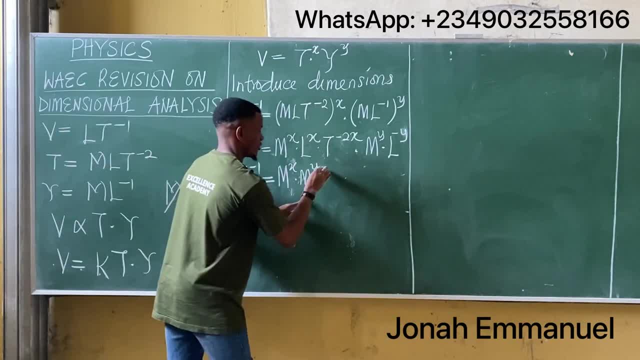 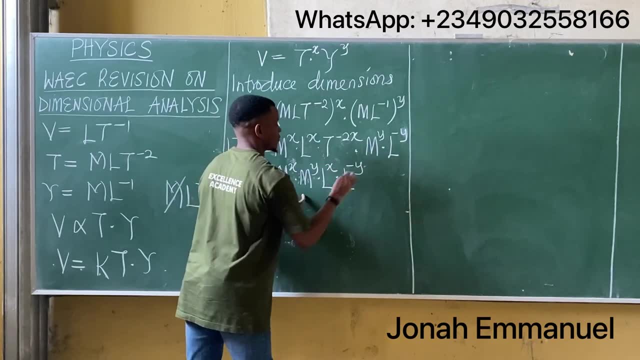 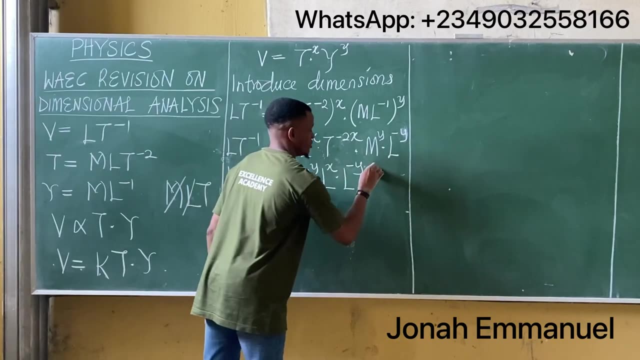 arrange the L's. So I have this one here. So it becomes L that's dot. L to the power X. dot this one here. L to the power minus Y. finally, arrange T's So dot. I have only one value for T So T to the power. 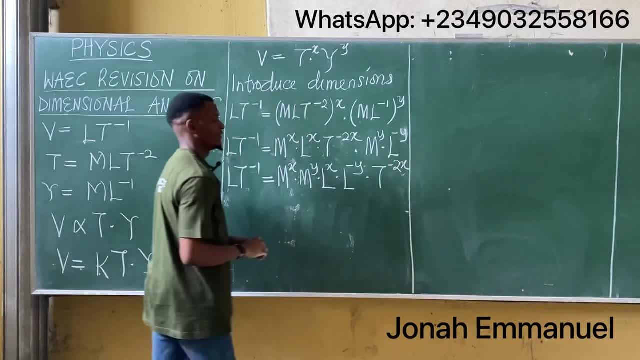 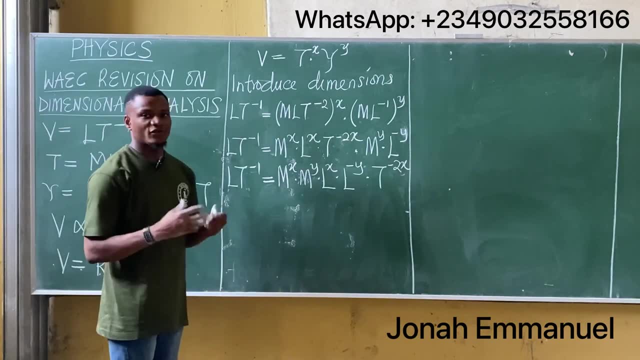 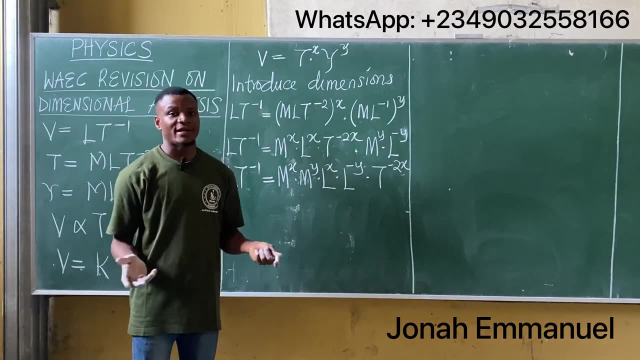 minus 2X, So I have this Alright. so, if you're done with this, our next task will now be using the idea of indices, which says that the index law says that if two bases- same bases- are multiplying, they add their powers. So hence I have 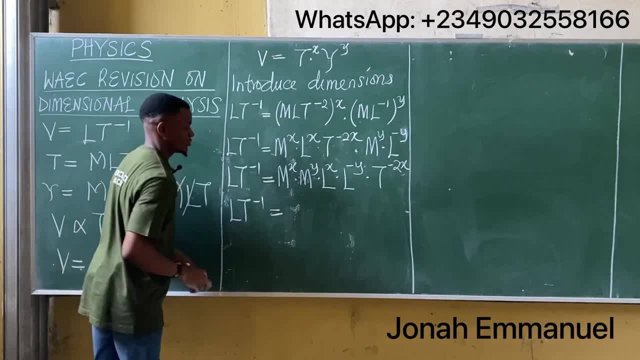 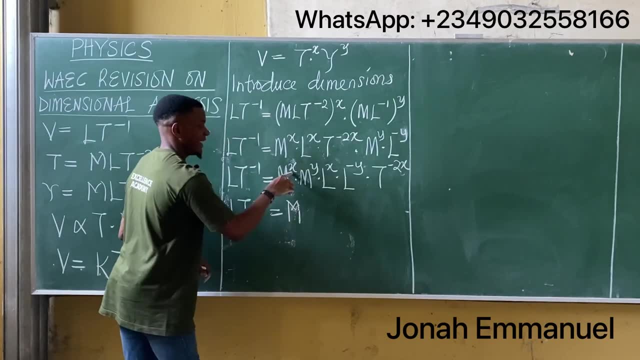 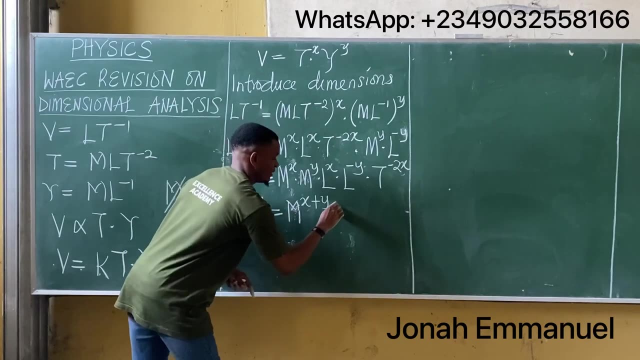 L, T to the power minus 1 is equal to. this is M and M multiplying. I will add up their powers So it becomes M into X plus Y. so X plus Y dot get L, So I have L. So it becomes X plus minus. Y Plus minus is minus. 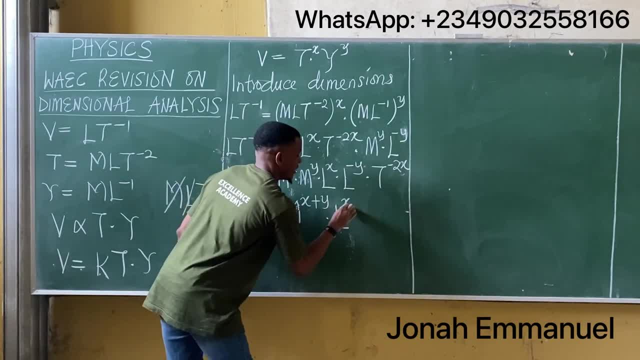 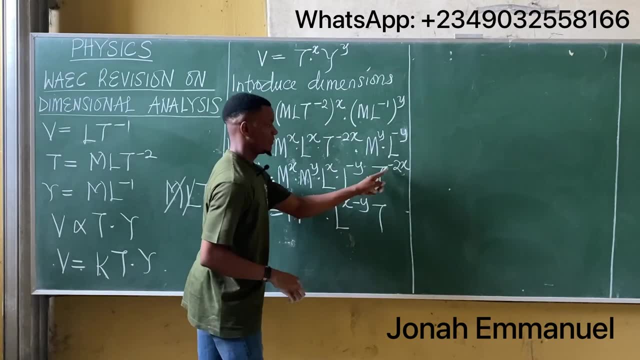 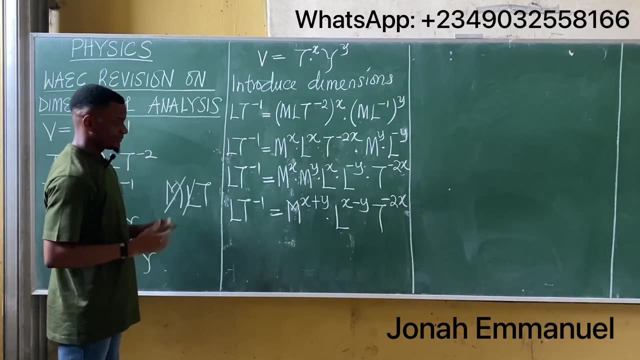 So it becomes X minus Y. I'm having X minus Y, And then I have T here, So it becomes T into minus 2X, So minus 2X. So I have this Alright at this point. now our next task will be to compare. 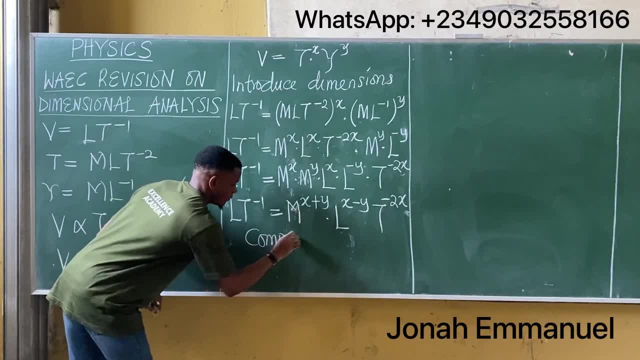 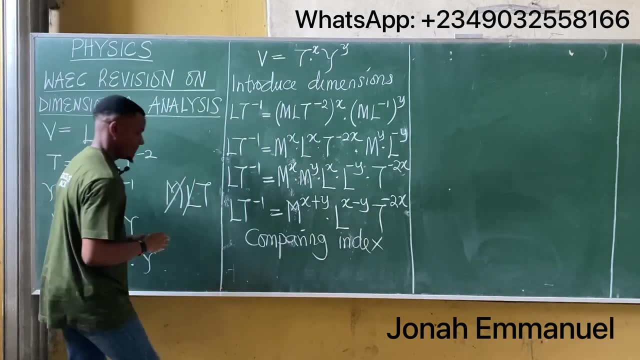 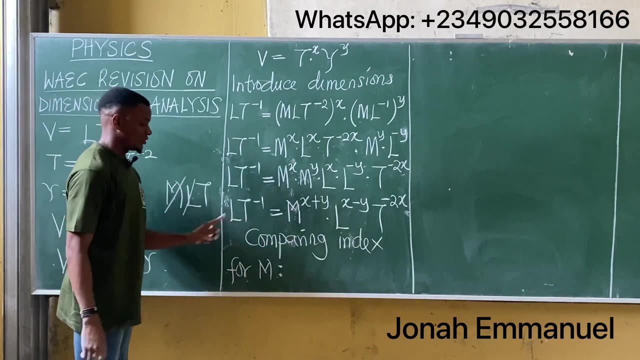 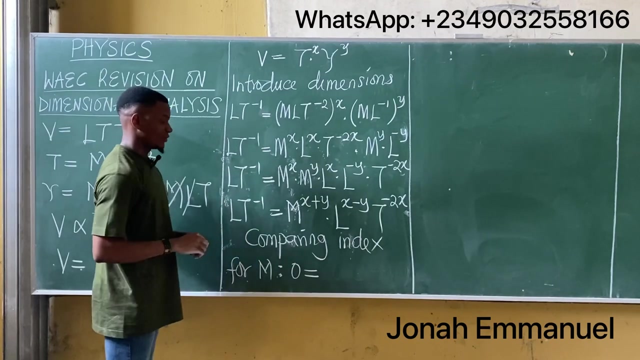 powers. Alright, so comparing index, So you can say index or powers, the same thing. Let's start with M For m. look at the left-hand part of the equation. There is no m, so it means the power is zero, equal. to look at the right-hand side of the 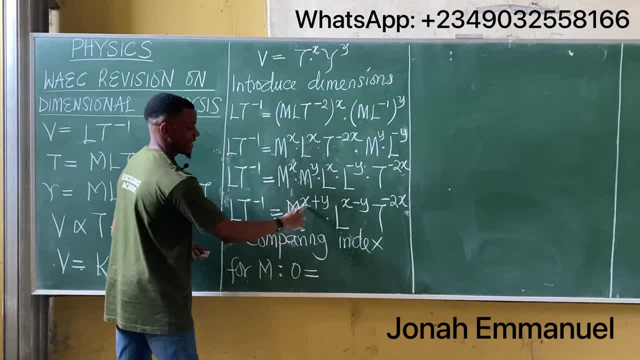 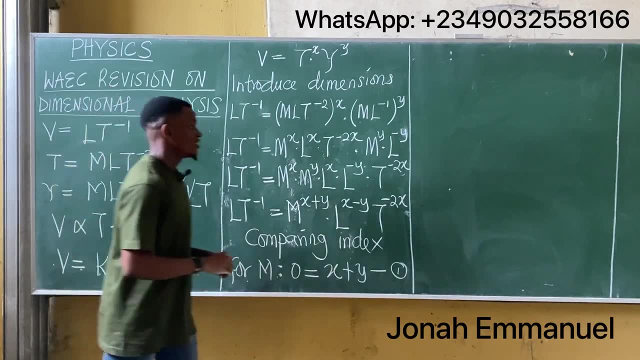 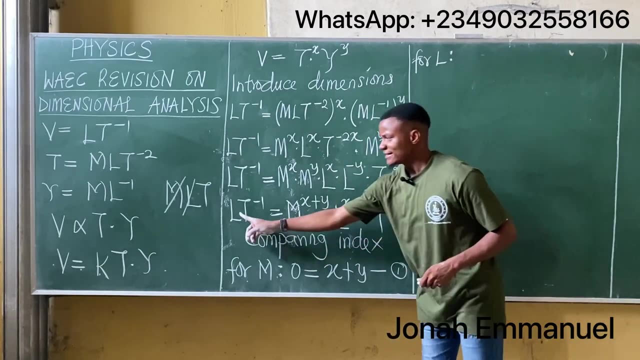 equation, which is this: You can see that the power of m here is x plus y, So I have x plus y. This is my first equation, Next up for l. for l, what do I have For the left-hand side of my equation? the power of l here is one. 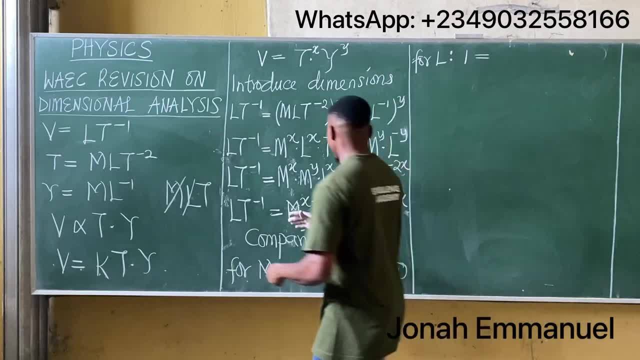 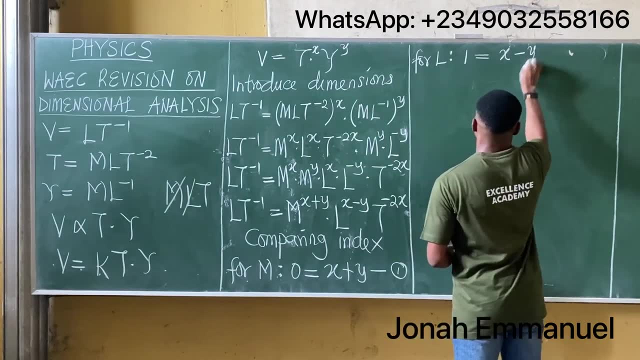 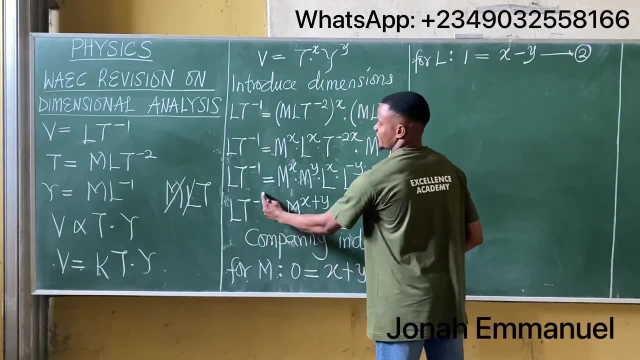 So I have one is equal to: for the right-hand side of the equation, the power of l is x minus y, So I'm having x minus y. Call this the second equation and then check for t, For t for my left-hand side, let's say for t for my left-hand side of the equation. 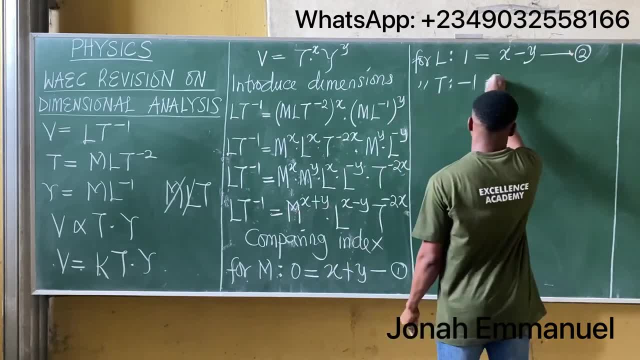 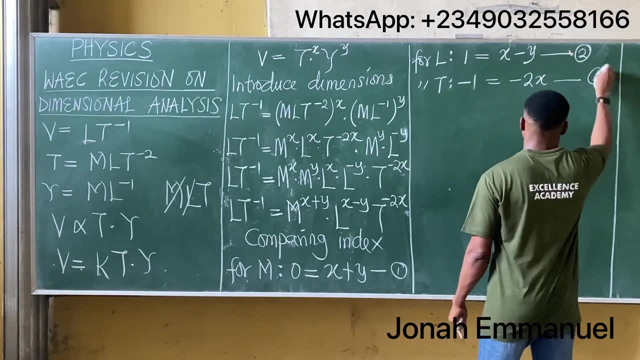 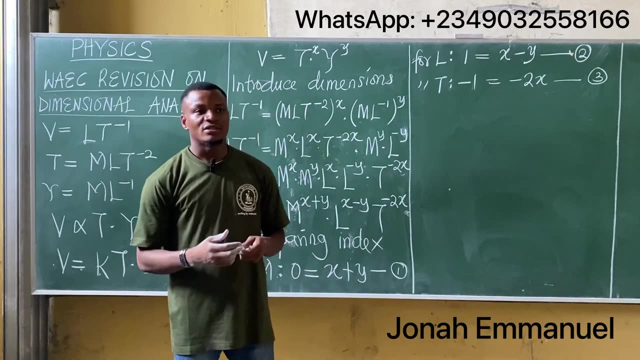 for t I have minus Minus one as the power being equal to for t. here the power is minus 2x, So minus 2x. This becomes my third equation. So when I compare the powers, I now have about three equations, sometimes four, depending. 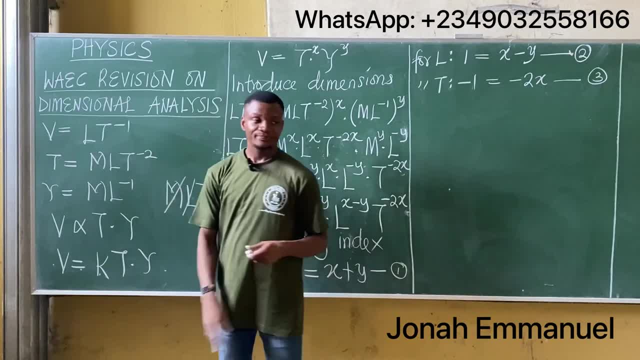 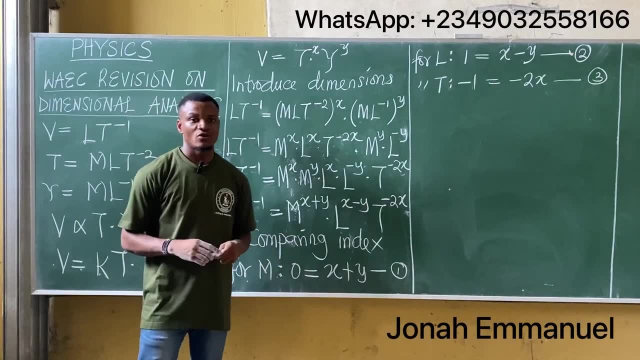 on the number of variables, I'm given Alright. So, having said that, what next? From equation one, two, three, we have, of course, in this equation we have two variables, which are x and y, So we have to find the value. 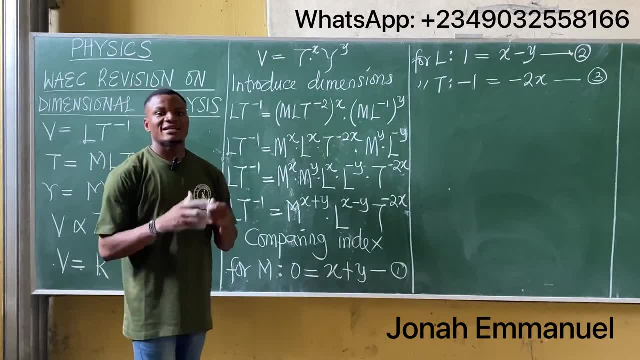 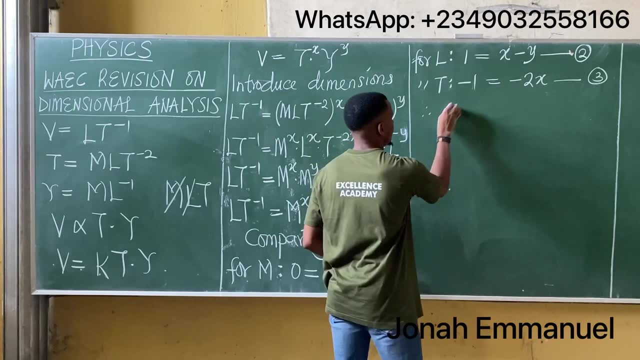 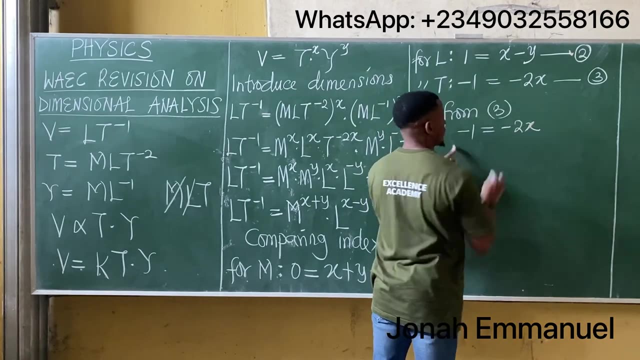 The value of x and y. From this, if you look clearly, there's an equation for which we can easily get x, and that's equation three. So therefore, from equation three we have that minus one is equal to minus 2x. 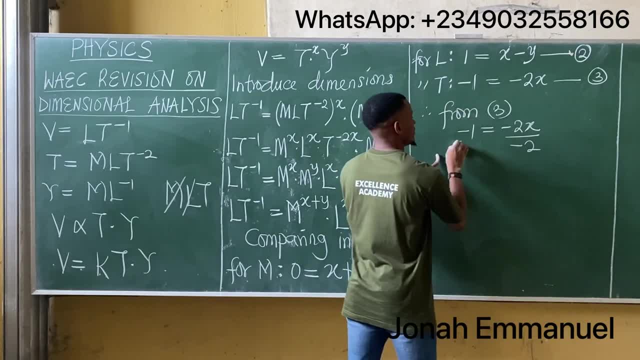 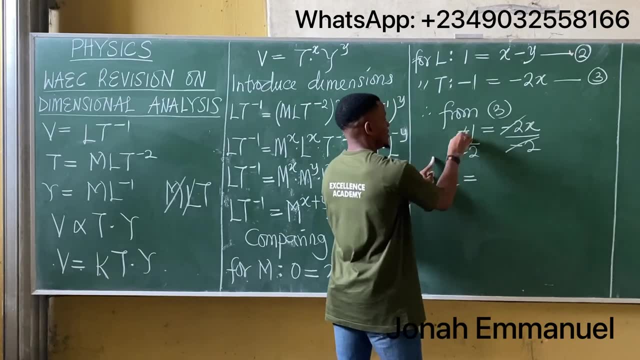 To get x, I'll divide here by minus two. divide here by minus two. This cancels this. I'm having x, So x is equal to this Cancels this. I have one over two. I've gotten the value of one over two. 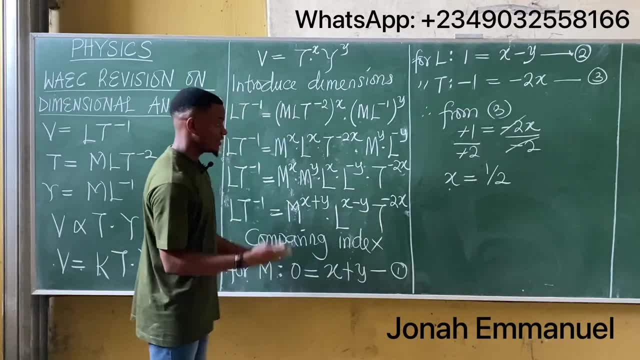 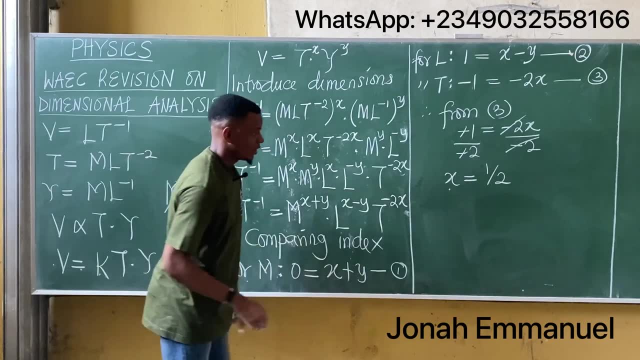 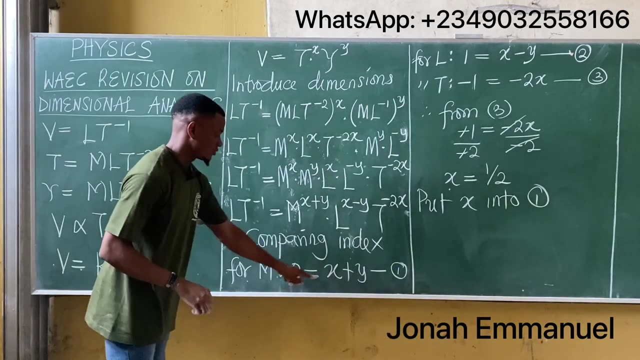 So my next task would be put the value of x either into equation one or equation two, and I'll have the value for y. Alright, let's use from one. So put x into equation one. From equation one, we have that zero is equal to x plus y. 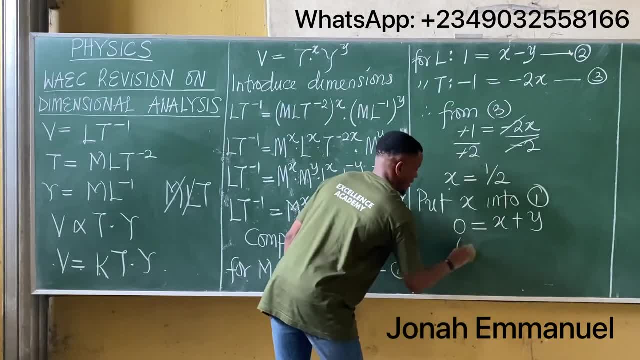 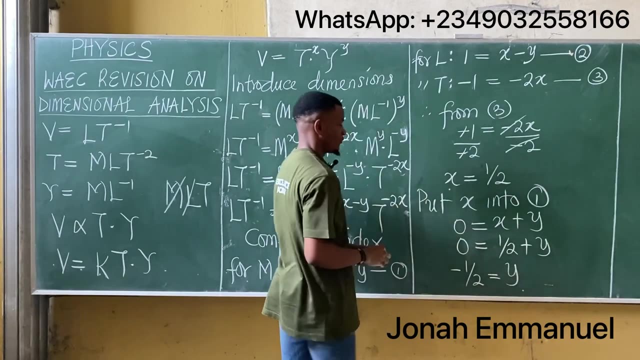 So x Plus y. Put x here, Zero is equal to x, is one over two plus y. Move this over here. So moving this is positive, Coming over here becomes negative. Minus one over two is equal to y. We've gotten x as one over two and y as minus one over two. 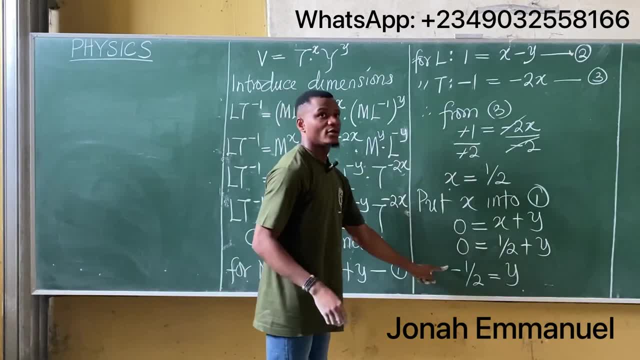 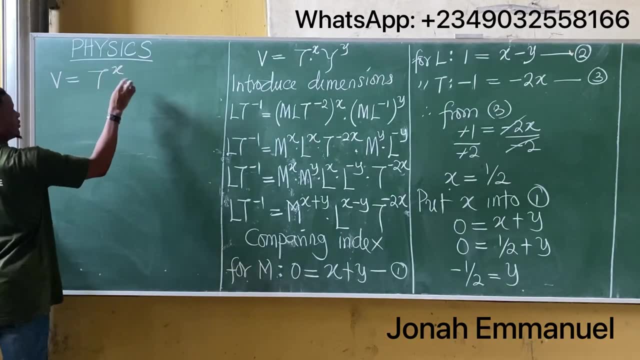 Alright, So I put the value of x and y In total. Let's put this equation here. So we said v is equal to t to the power x, dot gamma to the power y. That means v is equal to t to the power x. 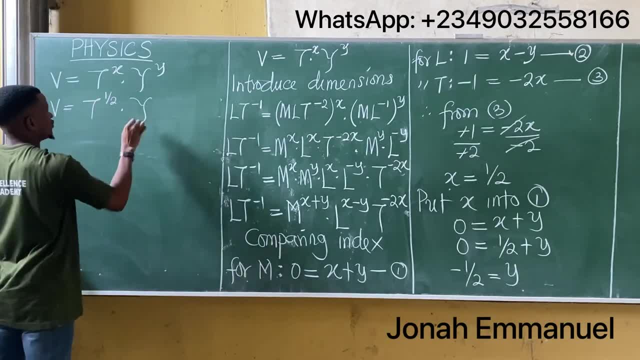 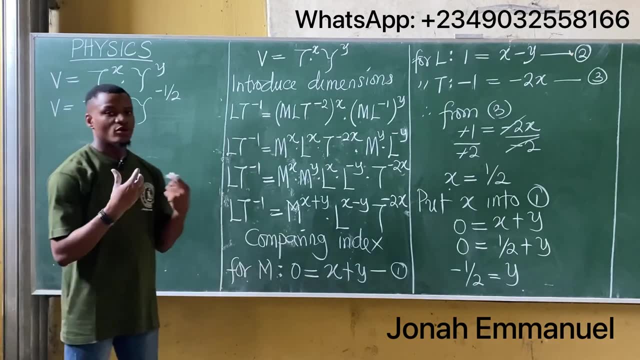 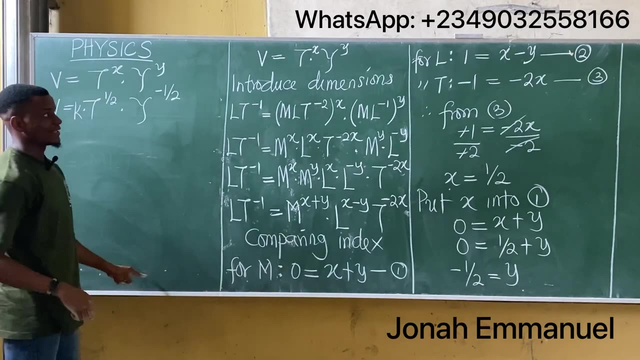 x is one over two dot gamma to the power y. y is minus one over two At this point now. you can now choose to bring in your constants if you want to. So you can add k dot here, Alright. So first of all you'll need your constant and do your solving. 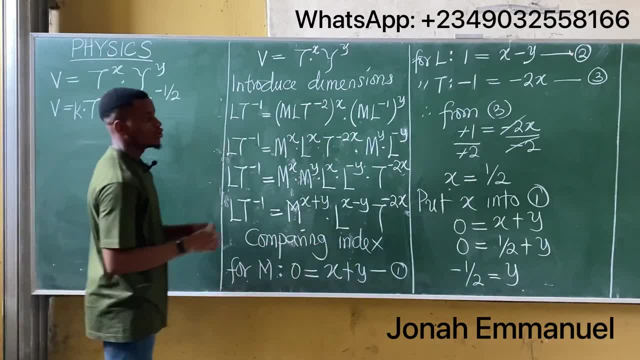 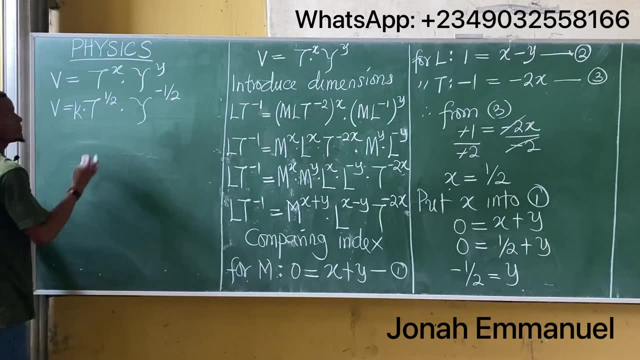 After solving, you now bring back your constant. That's, after you've gotten your value for your x and y, Bring back your constant. Alright, So we have this. Let's properly express this in mathematical sense. So v is equal to k, dot d to the power one over two. 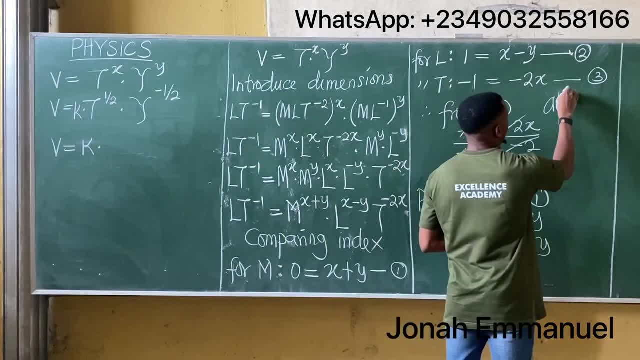 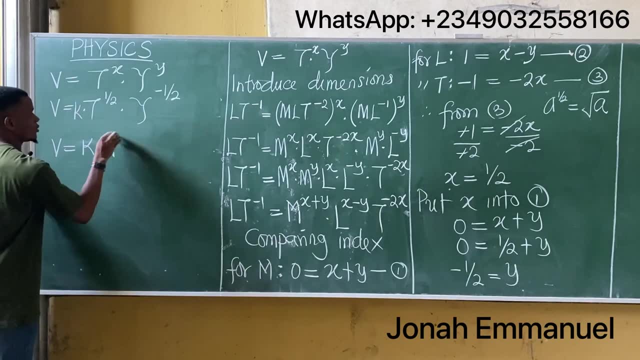 In indices we said a to the power. one over two is equal to two. Alright, to square root of a. so that means this becomes the square root of t tension dot. i'm seeing negative here. to eliminate the minus here i'll take inverse, so it becomes inverse of gamma to power. 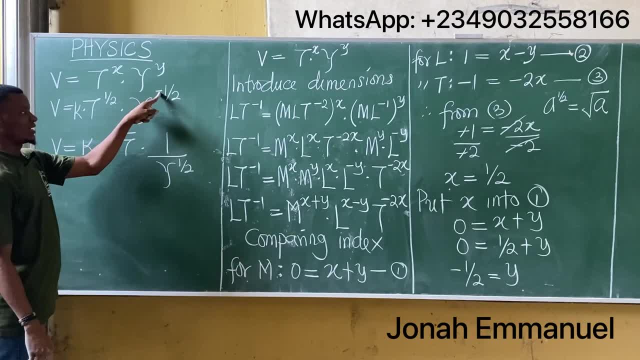 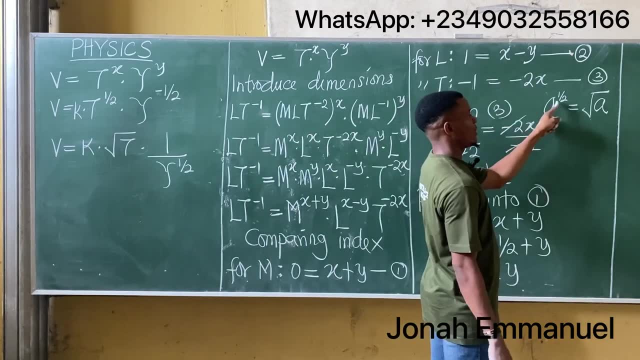 1 over 2. so to take out this minus here, i'll take 1 over, so i have this one here. all right, so we just said that if i have something raised to power 1 over 2, it's equal to the square root of that thing. 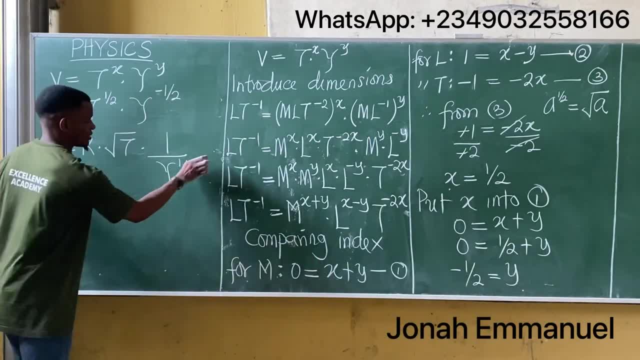 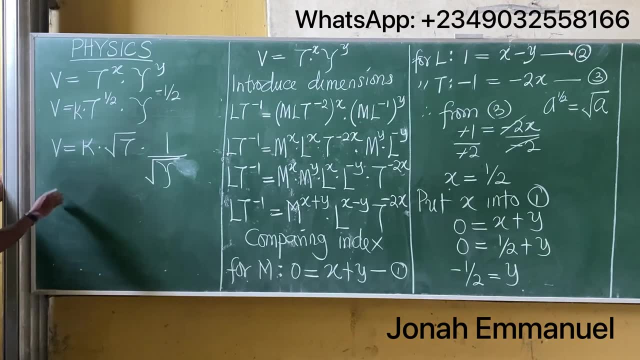 so hence this is equal to this becomes. i'll take this off and put the square root of gamma. all right, if i multiply this, v is equal to this times, this times 1, that's k root t, all over this root gamma. so i have this from the idea of indices we said. 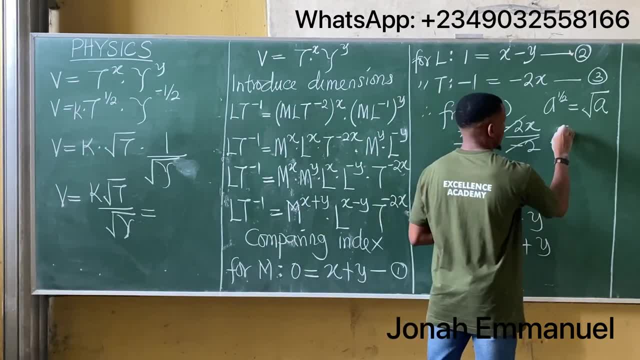 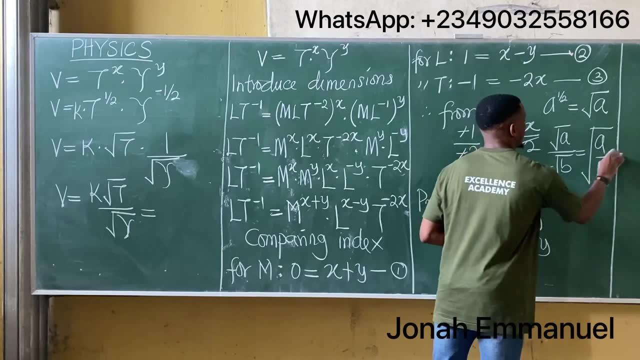 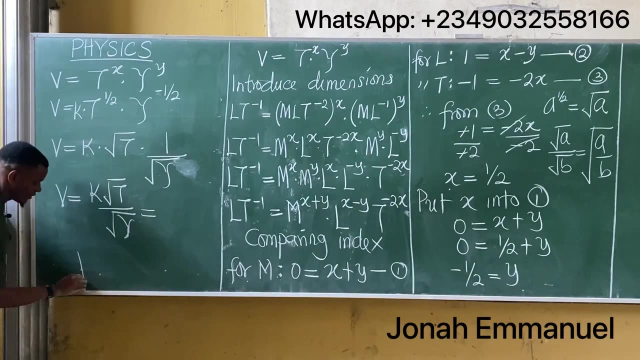 root a over root b is the same thing as square root of a over b, so i can put this in the same square root sign. if this is true, then it means that v is equal to k times the square root of tension c all over mass per unit length gamma. so i have this: 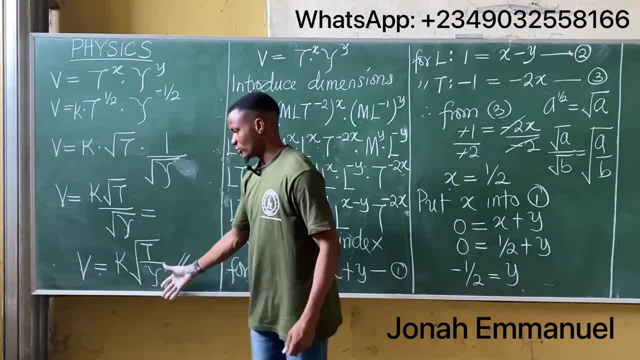 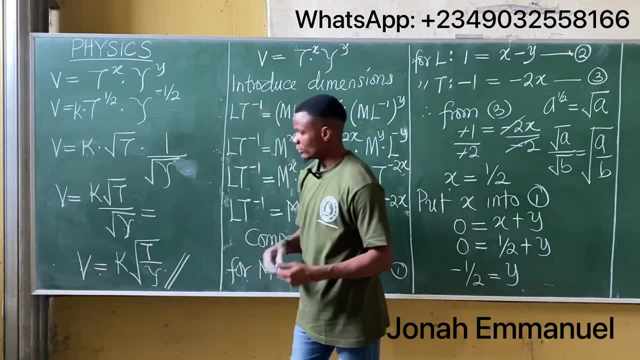 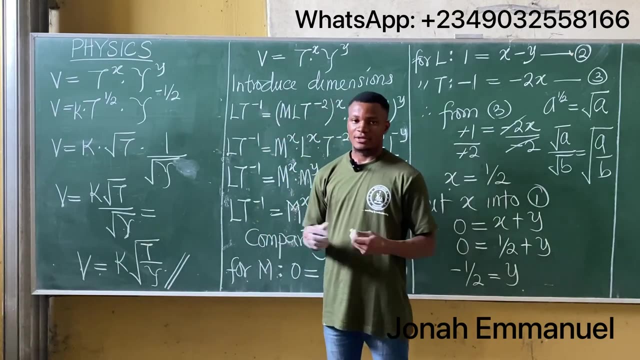 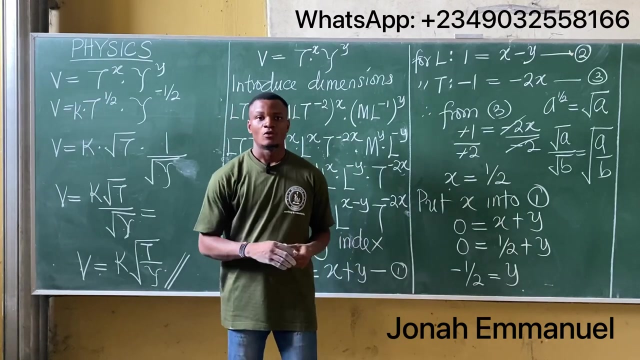 so this becomes the required relationship between the velocity, the velocity of the wave on the string, the tension on the string and the mass per unit length. so this is how we solve this question, um, if this is bulky. so this is how we solve this question. we've already done a full tutorial video.